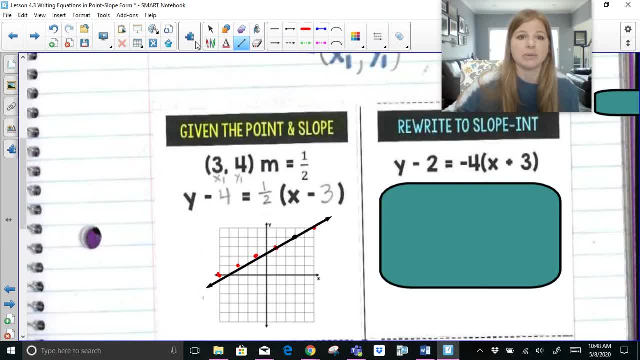 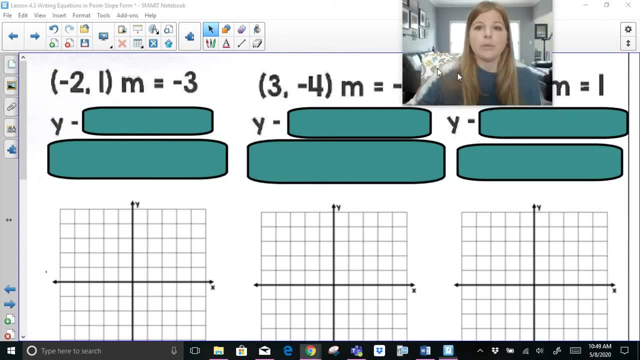 You see the point, You see the slope, You connect those up and you are Good to go. Let's try some more problems. We are going to write the equation. Let me just make my screen a little smaller. I don't know where to put me. 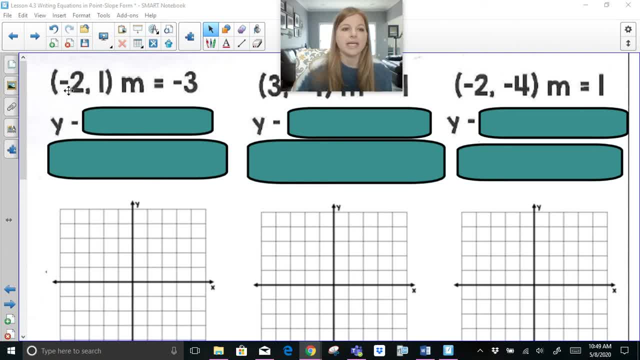 All right, We'll go over here. Negative 2,, 1, and then the slope is negative 3.. So it's y minus the y sub 1 value. So y minus 1 equals my slope of negative 3, open parentheses- x minus. 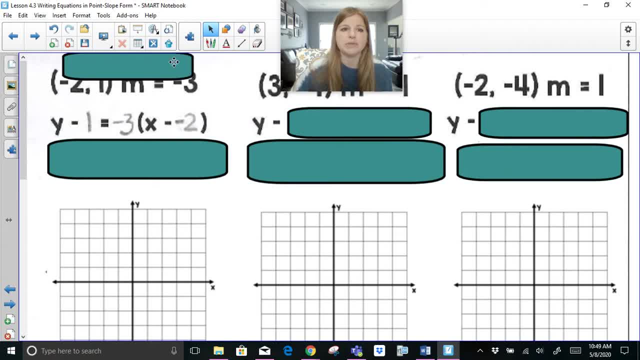 Now notice: my x coordinate is negative 2.. So I have to do x minus the negative 2.. Now let's clean this up a little bit. This would become: y minus 1 equals negative 3 times x plus 2.. Because we know, subtracting a negative means it's 2.. 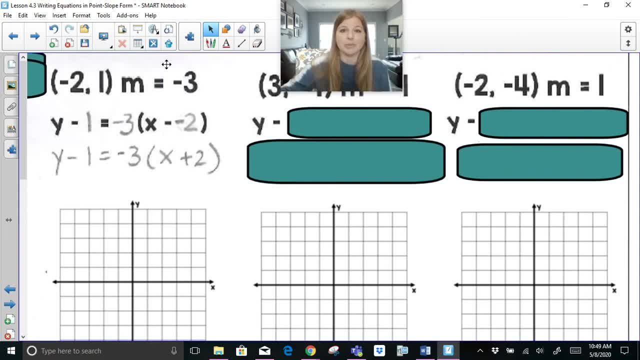 Now we don't distribute or anything like that. That is truly what point-slope form is. So I'd go ahead. I'd be able to plot my point of negative 2, 1, and plot my slope of negative 3.. 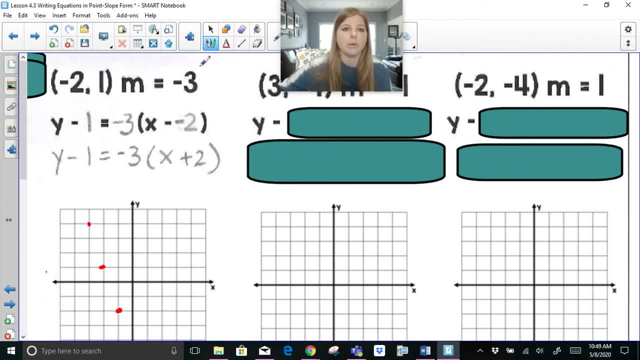 Down 3 to the right 1, down 3 to the right 1, or up 3 to the left 1.. And there's my line. Pretty nice, Okay. Let's take a look at the next one. So the formula is y minus the y value. 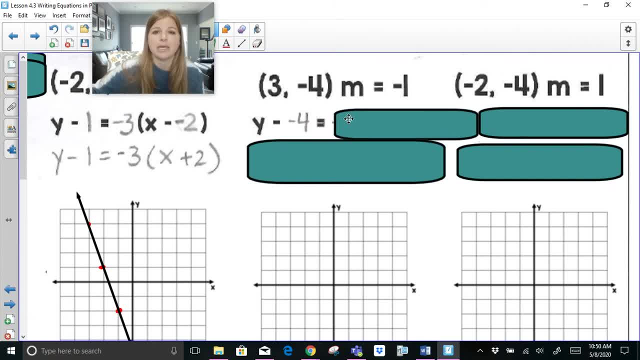 So y minus negative 4.. We're going to have to clean this one up as well. Equals the slope negative 1, times x minus my x value of 3.. We know y minus the negative 4 really means y plus 4.. 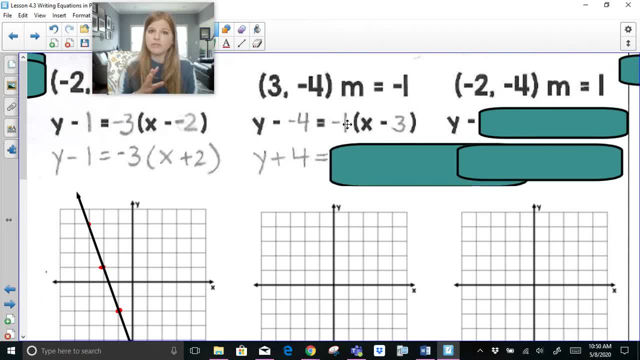 The other special thing is that we don't need to put a negative 1 in front of our parentheses, but we do still need the negative. It's like when you don't write negative 1x, you just write negative x. It's kind of the exact same idea. 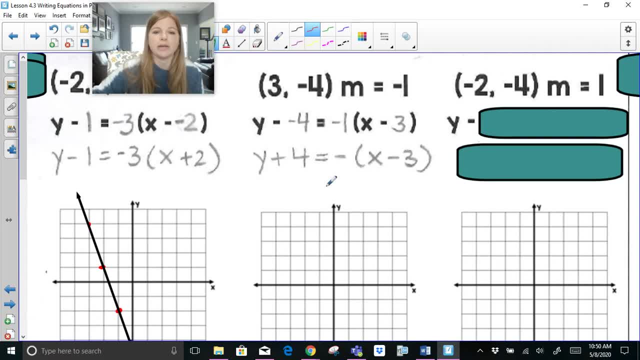 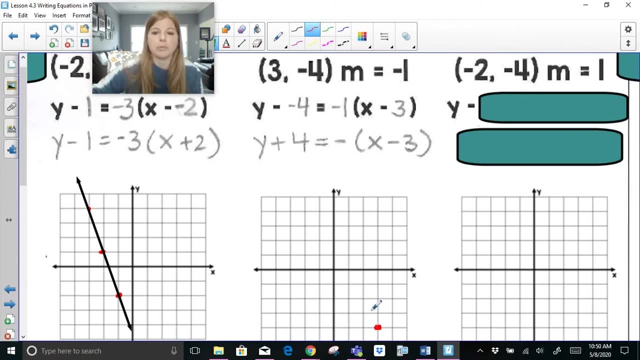 And the rest is pretty good. If I wanted to go ahead and graph this, I'd plot my point at 3, negative 4.. So that's right here. A slope of negative 1 would be down 1 to the right, 1.. 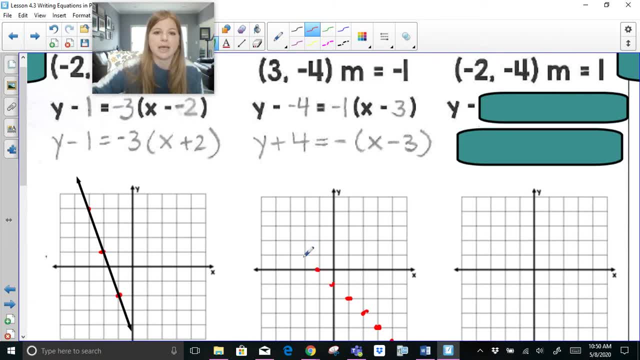 I can go backwards And I have my graph Pretty good, All right. Last one of this scale. So y minus the y value of negative 4 equals my slope of 1 times x minus the x value of negative 2.. So lots of things going on here. 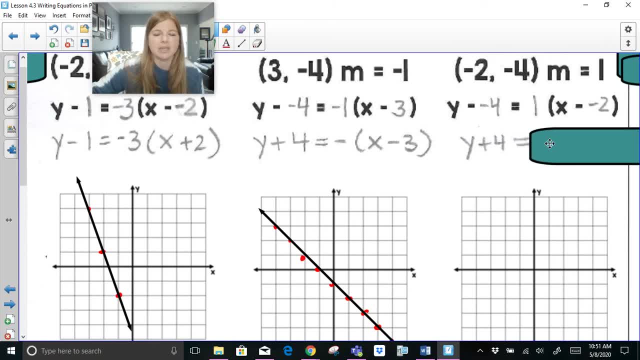 y minus the negative 4 really means y plus 4.. If it's 1,, I don't need the 1.. And then if I don't need the 1,, then I don't even need the parentheses, So it actually just still becomes x plus 2.. 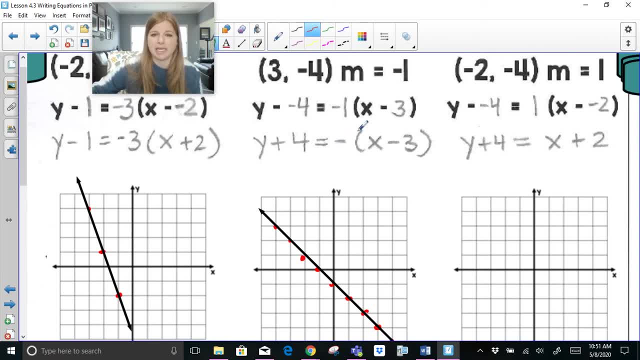 So. So I needed the negative here, because it's got to be negative the entire value and I'm not distributing anything, But having a 1 in front is pretty unnecessary, And then the parentheses aren't needed anyway. Negative 2, negative 4, a slope of 1.. 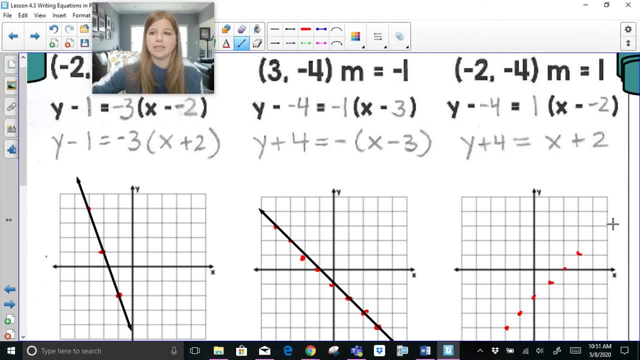 And this is what my graph should look like. So working in point-slope form, writing the equation, is pretty easy. We just have to watch our signs And then we need to clean anything up, And then we just plot the point. plot the slope. 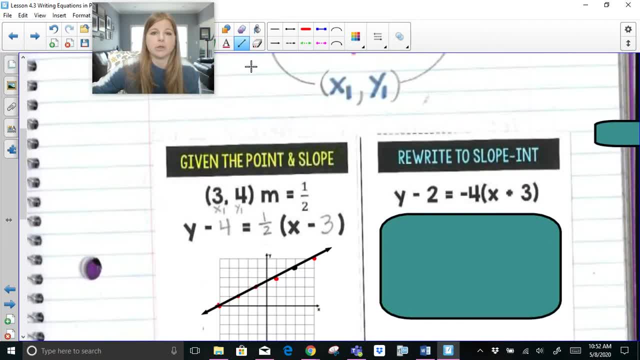 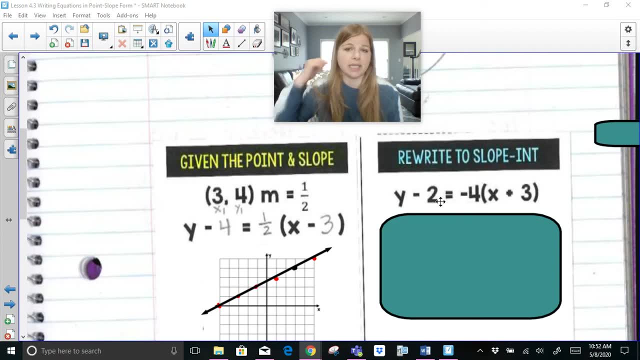 Let's take a look at our next skill: Rewrite to slope-intercept form. So here I have this equation that is definitely in point-slope form. My point, if you can see it, is negative 3, 2. Because it's the opposite of this x value, and then this 2 here. 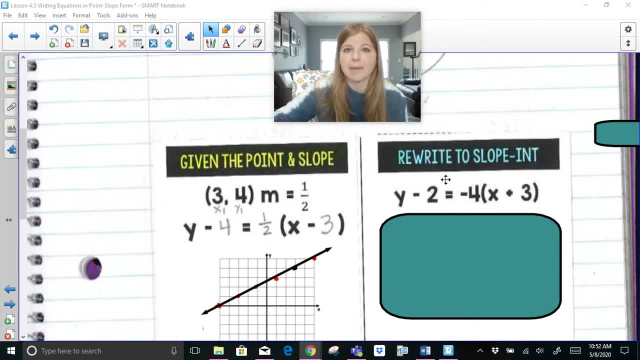 My slope is negative 4.. Slope-intercept form is: y equals mx plus b, So I need the y to be by itself. First thing, basically, That should be kind of screaming out to you, Is that we definitely need to do the distributive property. 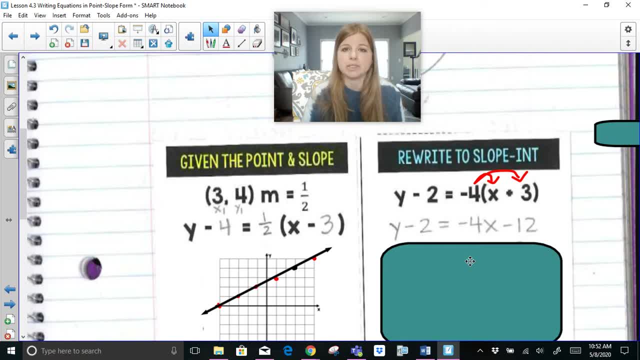 So if we distribute that out, we end up getting y minus 2 equals negative 4x minus 12.. And then the last thing would be to get y by itself. So I would go ahead and add 2 on both sides And I would end up getting y equals negative 4x minus 10.. 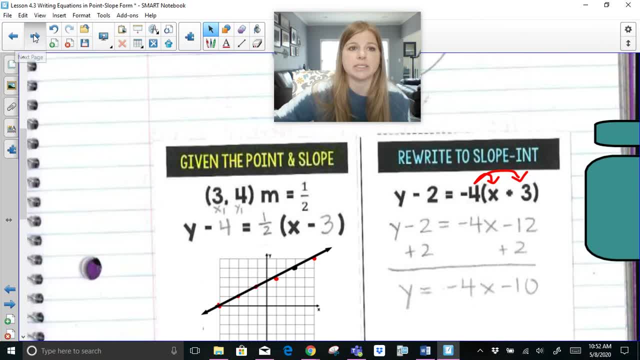 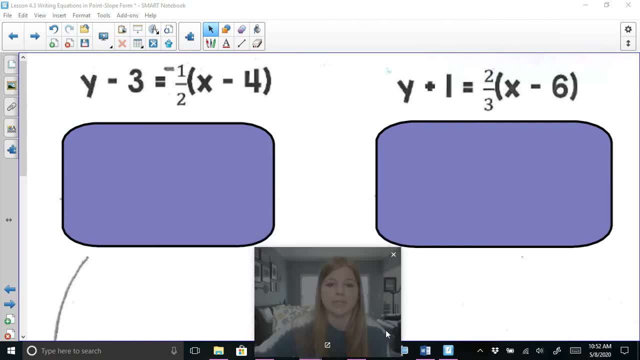 Pretty good, So rewriting into slope-intercept form really isn't too bad at all. Let's take a look at these two problems here. Okay, All right. So if I wanted to put these in slope-intercept form, I would first distribute. 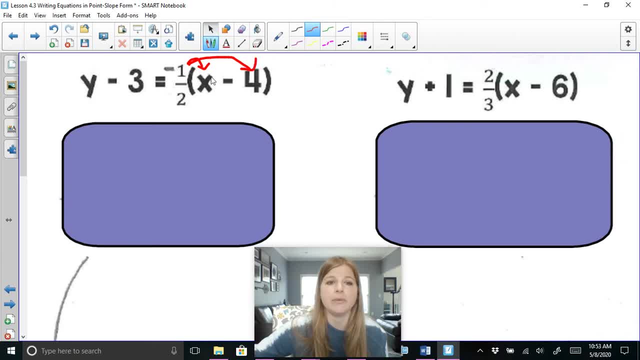 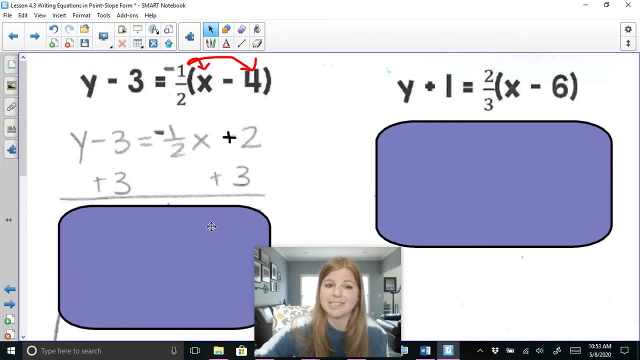 So negative 1 half times x, negative 1 half times negative 4, which becomes y minus 3 equals negative 1 half x plus 2.. And then simply add 3 on both sides And we get y equals negative 1 half x plus 5.. 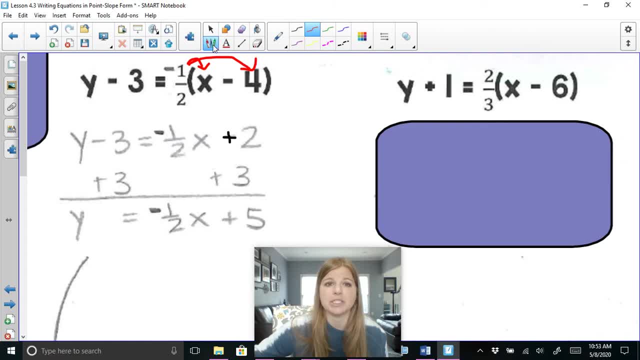 Same thing over here. If I wanted to start to get this next equation into slope-intercept form, I would distribute my 2 thirds, So this becomes: y plus 1 equals 2 thirds x. 2 thirds of 6 is 4.. 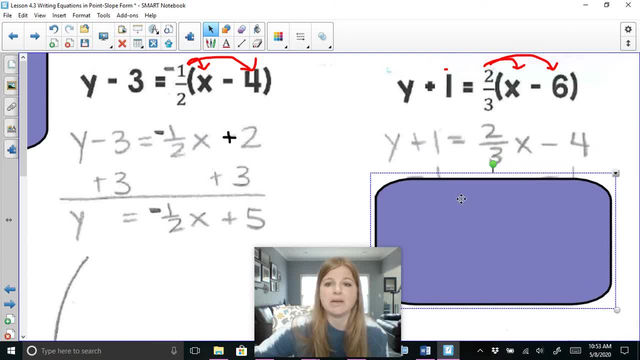 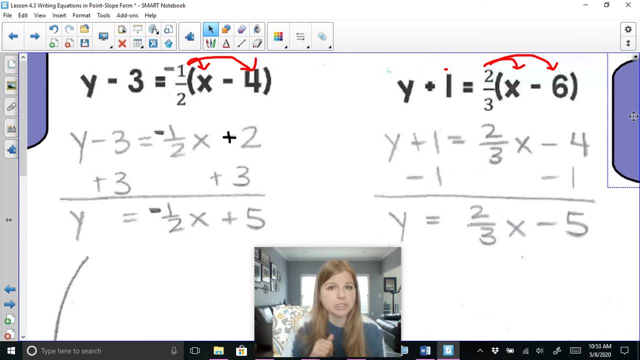 So that becomes minus 4.. And then to get y by itself, I would subtract 1 on both sides. I get y equals 2 thirds x minus 5.. So I can write an equation in point-slope form. I can graph it. 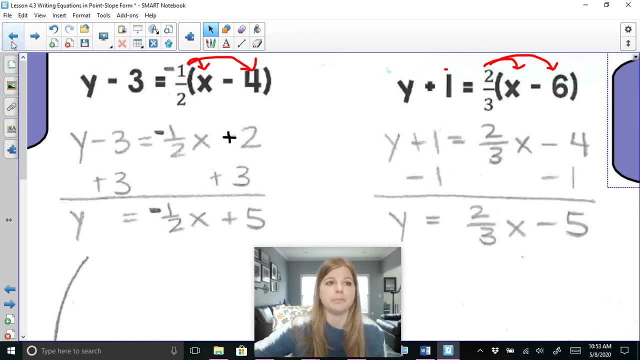 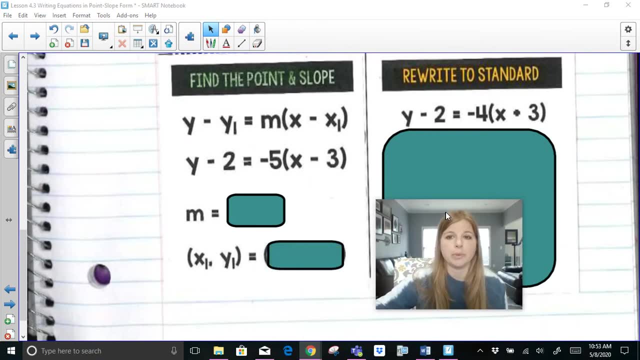 I can also rearrange the equation into slope-intercept form. Next skill for us, The next skill we're going to take a look at, is to find the point and the slope. So just by looking at an equation that's in point-slope form, 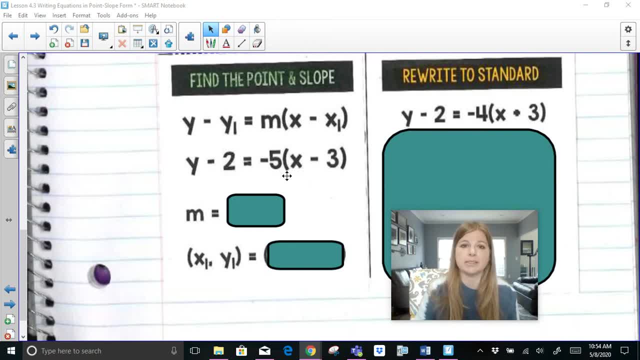 I want to be able to see what the slope is and see what my point is. So here in this equation, I think it's pretty obvious that our slope is negative 5, because it's the number that's right in front of our parentheses. 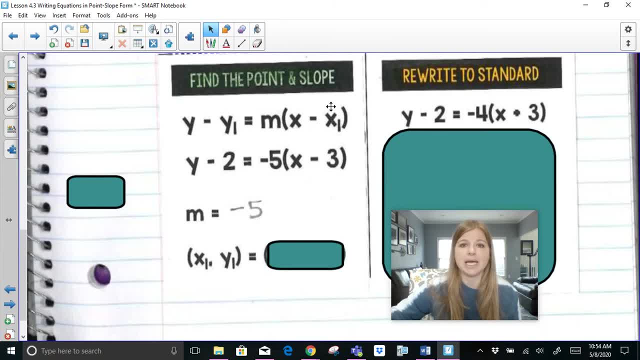 Our x and y value. now remember it's x minus the x sub 1.. So here, if I see x minus 3, that means my x sub 1 is positive, 3. If I see y minus 2, that means my y value was. 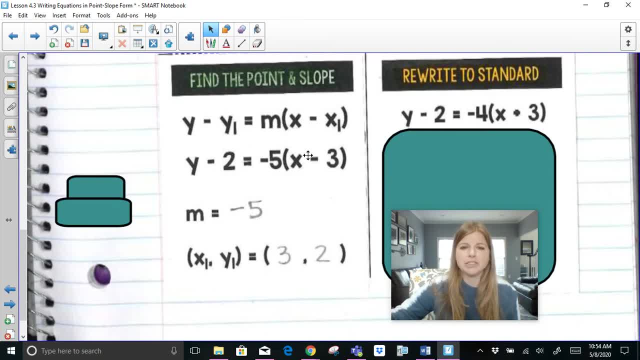 positive 2.. Pretty nice. Now imagine this said x plus 3.. If it said x plus 3,, the only way to get x plus 3 is if this said x minus a negative 3.. And if it said x minus negative 3, then we really know that becomes x plus 3.. 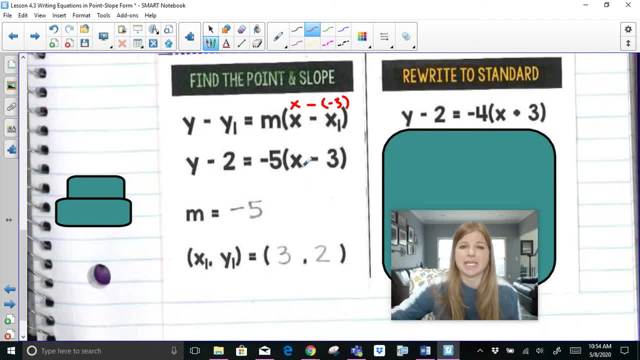 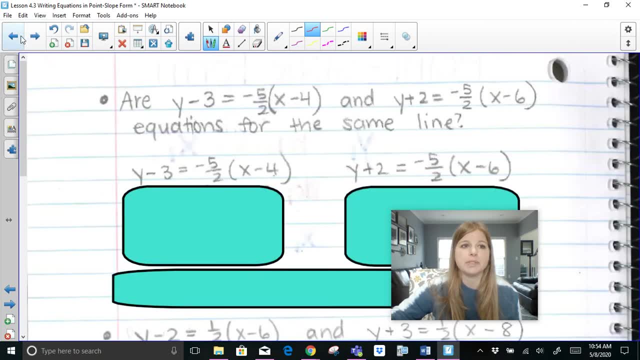 So that's the only way that this would be negative if that was the case, if this said: x plus 3.. So let's try these next couple problems of that skill: Oops, Okay, All right, Let's see what we can do. 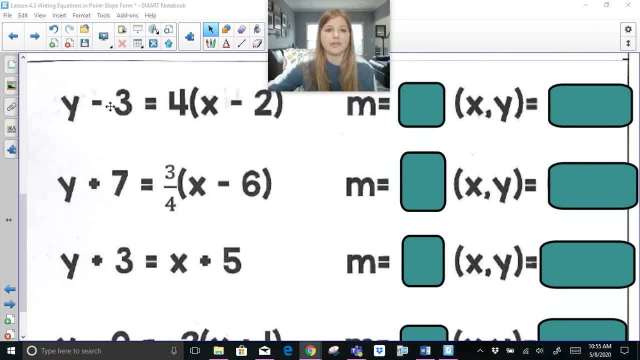 And now I keep moving my screen around. Okay, first equation: y minus 3 equals 4 times x minus 2.. I think it's pretty clear. our slope is 4, because it's always this number in front of the parentheses. If it's x minus 2, my x value is 2.. 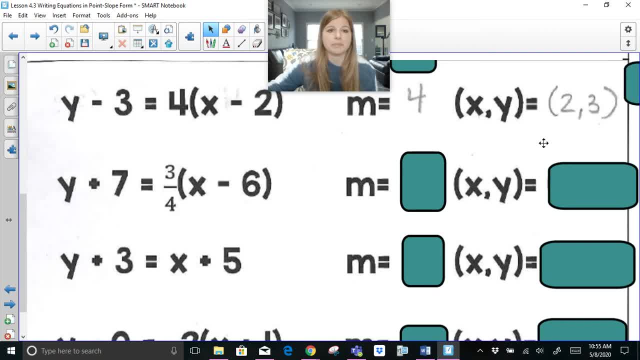 If it's y minus 3, my y value is 3.. The next one: my slope is 3 fourths. Again, I always think the slope is 3 fourths Slope is the easiest thing to find. It says x minus 6, so my x value is 6.. 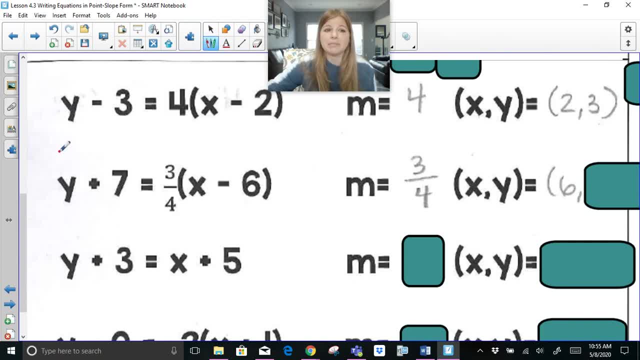 y plus 7.. y plus 7 means it's y minus a negative 7.. That's the only way to get y plus 7 in this formula, So my y value is actually negative 7.. Let's take a look at the next one. 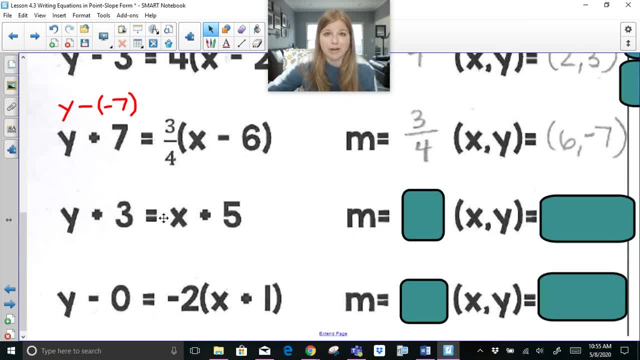 I don't see any parentheses or a number in front of the x. but there really is a number there, It's just 1.. So that would be a slope of 1.. If I see x plus 5, that really means it's negative 5.. 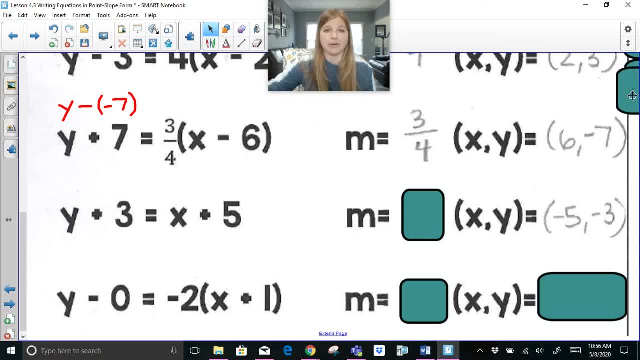 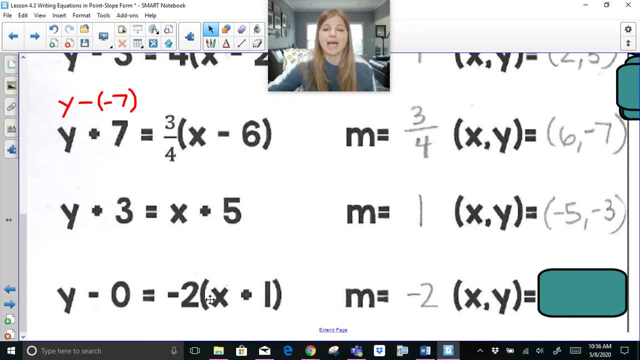 And y plus 3 means the y value would be negative 3.. Good, Last one. My slope is negative 2.. If I see x plus 1, that means my x value is negative 1.. And then y minus 0 would mean that my y value is just 0.. 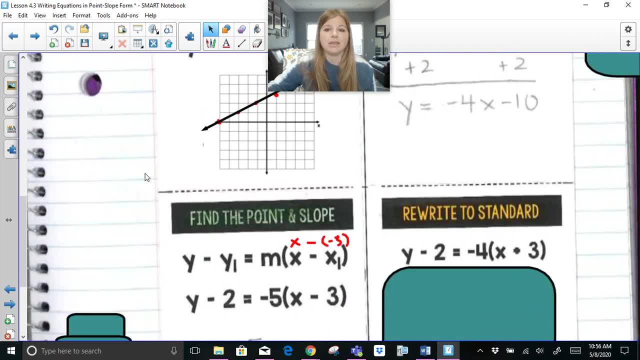 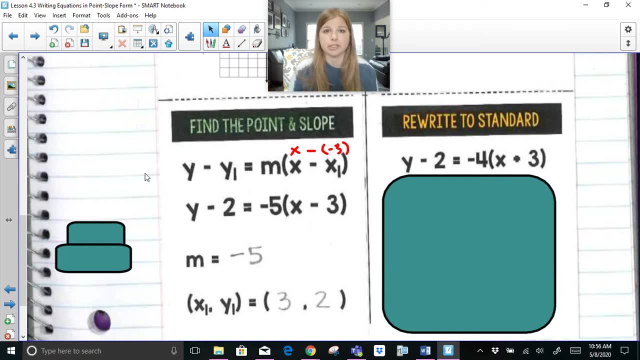 Pretty good. Last skill: Rewrite to standard form. So we did a previous part in this lesson where we rearranged it into slope intercept form: y equals mx plus b. But now we're going to take a look at this equation and put it into standard. 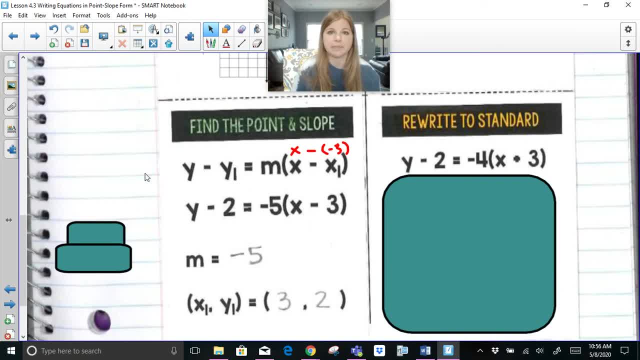 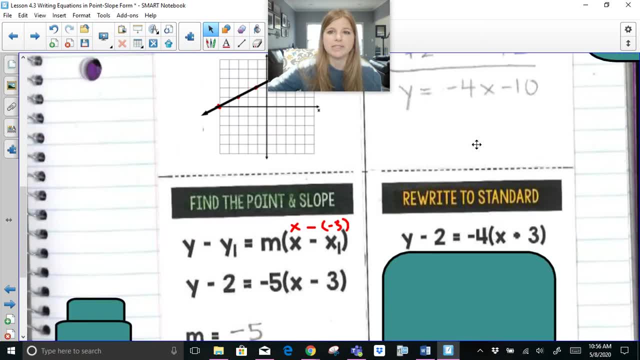 Standard form is ax plus by equals c. Now, in order to actually do that, to get it in that form, I really need to do all of the same steps I did here To make it look like ax plus by equals c. I still need to distribute. 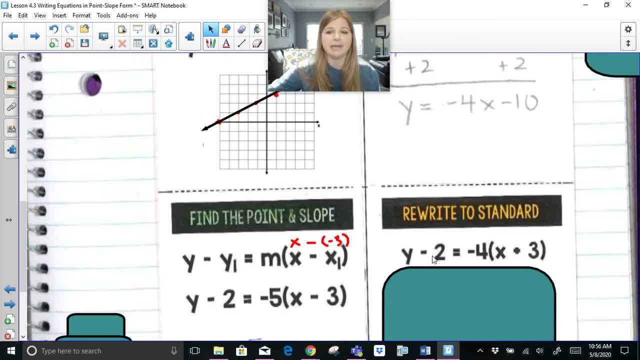 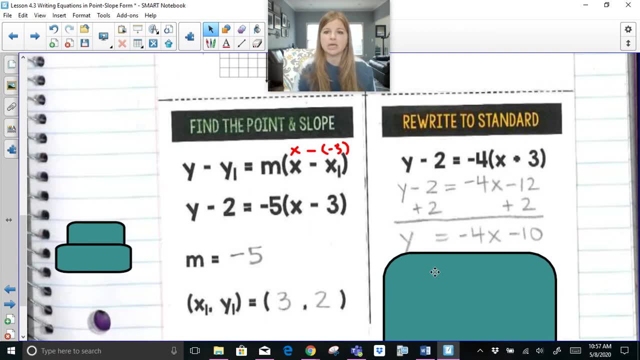 I still need to send my constant Over to the right hand side, And I really would at least need to start off by putting this equation into slope intercept form first. Now rewriting this into standard happens in just one for this case. one nice step. 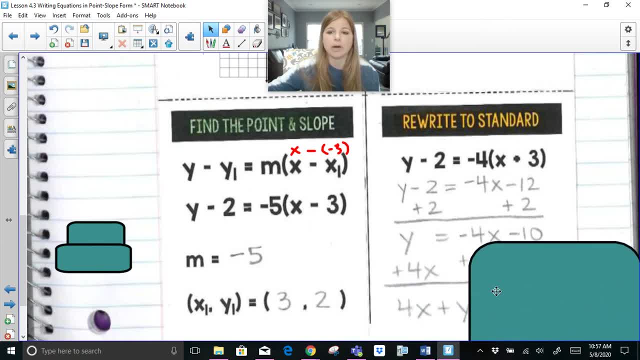 It would be to add 4x on both sides, And now I get 4x plus y equals negative 10. Ax plus by equals c, And it's exactly in the order that I need it to be in, Which leads us here. 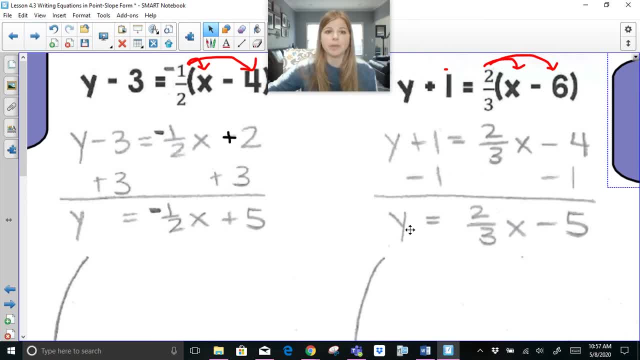 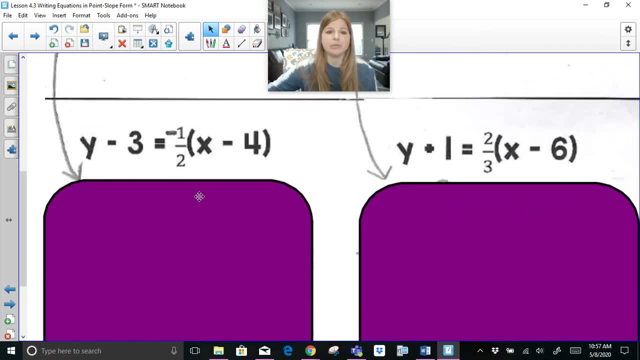 We rewrote these equations into slope intercept form, But now let's take these equations and write them into standard form. So we're going to do ourselves a favor and we're not going to rewrite everything um that we had from before. 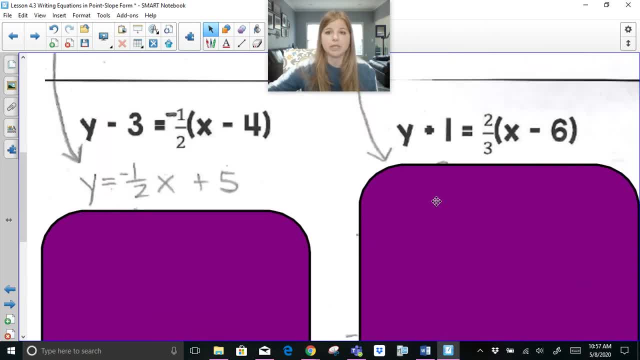 We're simply going to continue these equations with what we put into slope intercept form. So now let's think about it. If I need this equation to look like ax plus by equals c, I would need to add 1 half x on both sides.